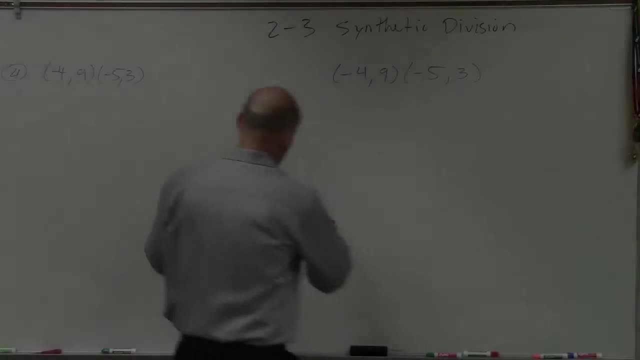 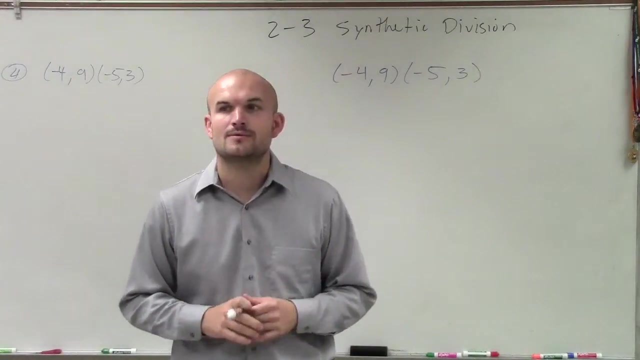 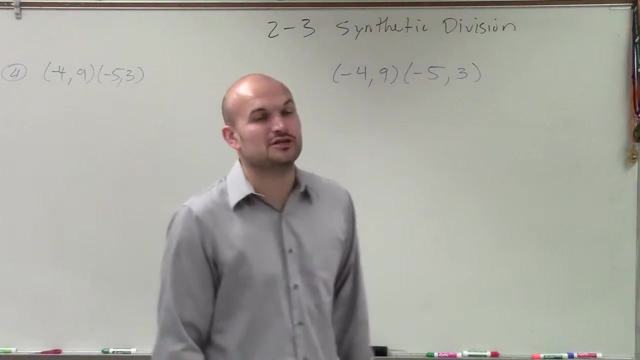 Subtitles by the Amaraorg community. So here we go. So, anyways, I'm going to ask you, ladies and gentlemen, to be able to determine the points, the distance between these two points, and they're not graphed. One thing we want to label is: 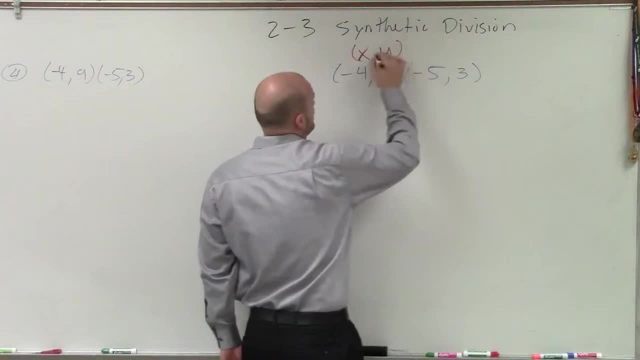 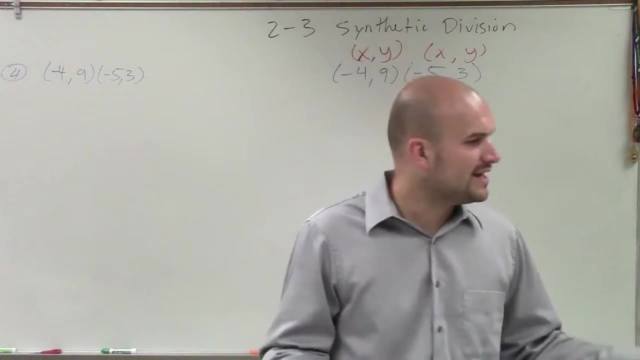 remember, every point comes in the form of xy. right, Every point can label as an xy. but, ladies and gentlemen, we have two points, So I need some way to distinguish between point number one and point number two. So what I do is I use these nice little subscripts. 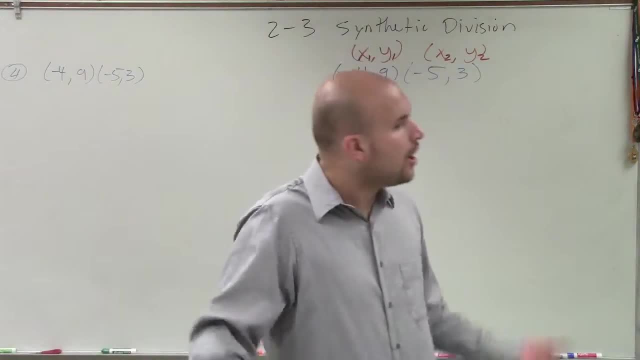 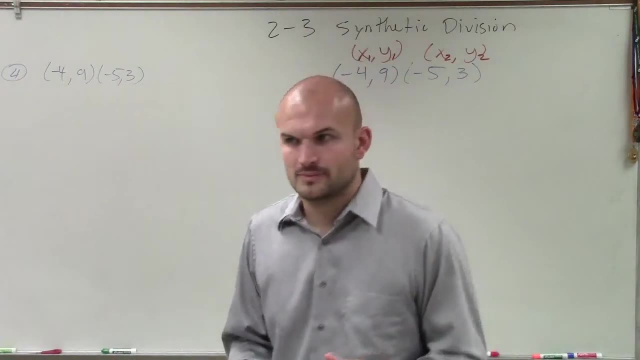 x1, y1, x2, y2.. All it is is a way to label them. The one and the two don't have any numeric value with the points. They're just a way to label them. Okay, Now let's go ahead and take a look. 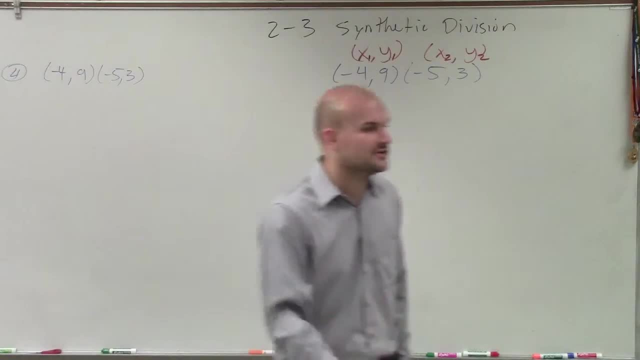 at the distance formula. Now, this is something I've been trying to present to you that you're going to want to make sure you have written down, which we're going to talk more about on Monday as well, But if I want to find the distance between two points, 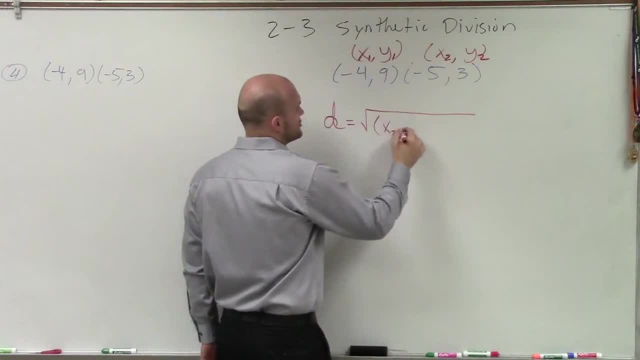 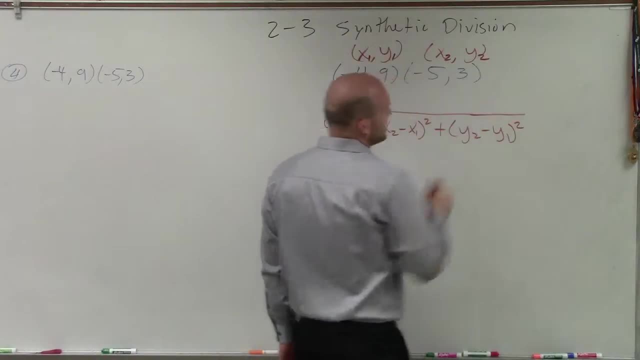 that becomes the square root of x2 minus x1 squared plus y2 minus y1 squared Again, don't worry so much about this formula. We're going to talk more about where it comes from again, But right now I just want to make sure. 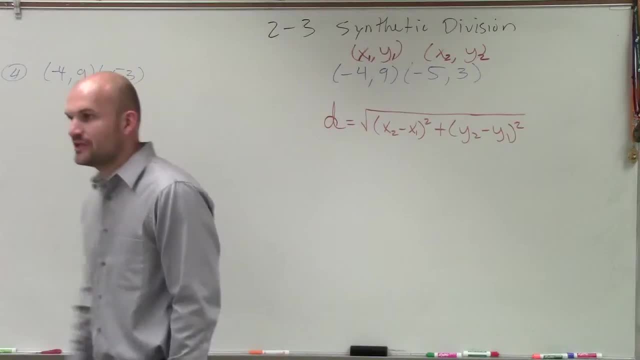 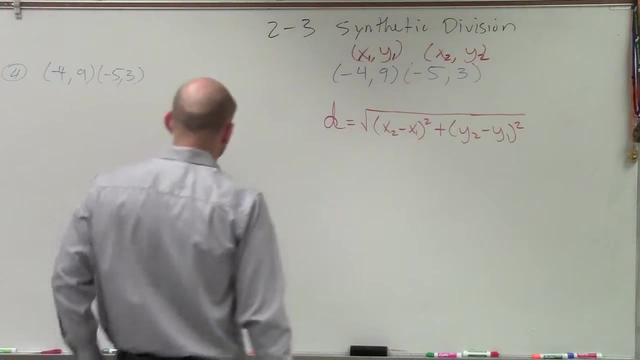 that everybody has that formula in their notes so they can apply the problems that we're going to be working on today. Because in label now, what we're simply just going to do is- let me give you guys an example, If you guys remember, 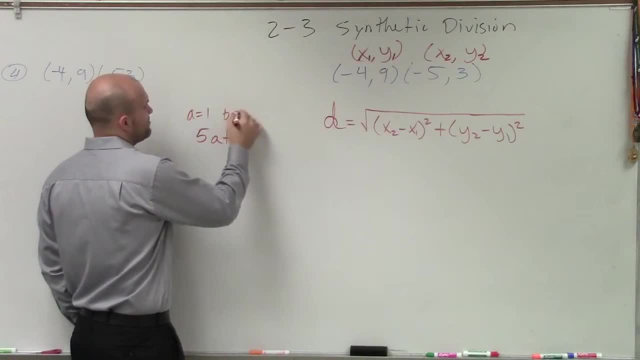 if I gave an expression 5a plus b and I said a equals 1 and b equals 3, what do you do with the 1 and the 3?? Do you remember what you do with 1 and the 3?? 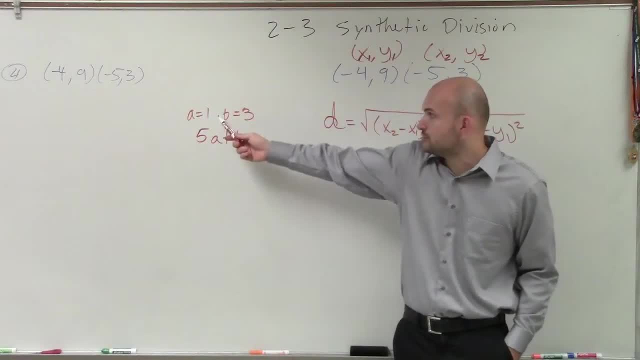 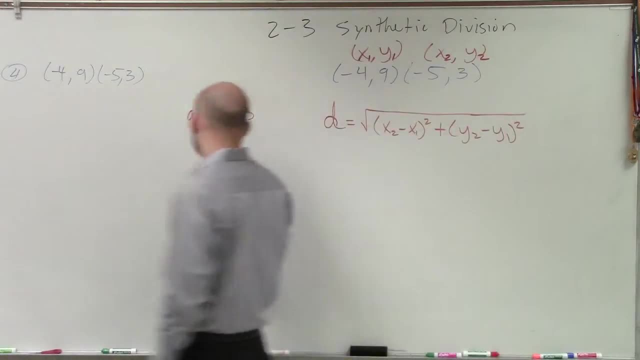 If I said: simplify or evaluate this, what would you do with 1 and the 3?? You'd plug it in for the a and the b, right. Good If I said: f of x equals x plus 5, and then I say: fine, f of negative 1,. 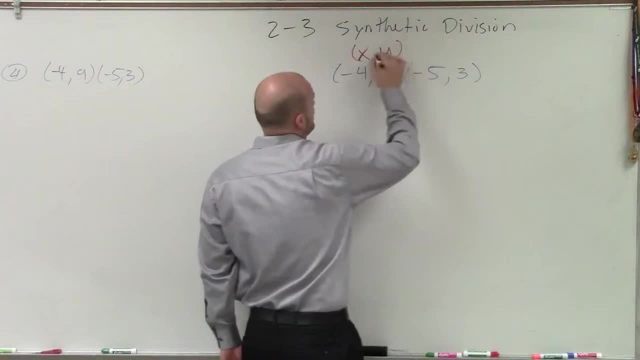 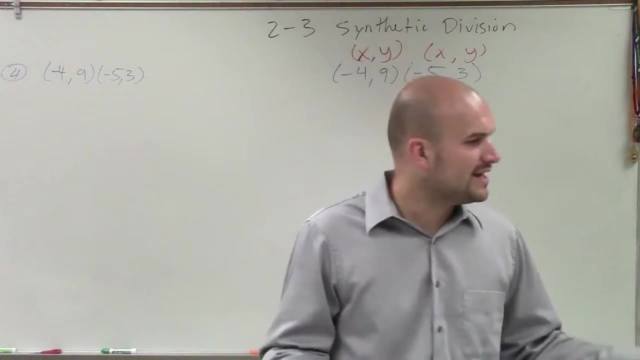 remember, every point comes in the form of xy. right, Every point can label as an xy. but, ladies and gentlemen, we have two points, So I need some way to distinguish between point number one and point number two. So what I do is I use these nice little subscripts. 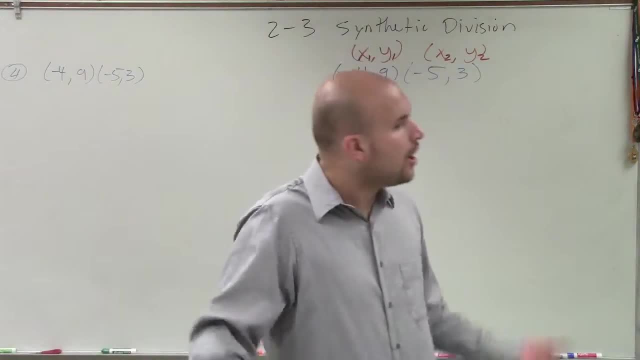 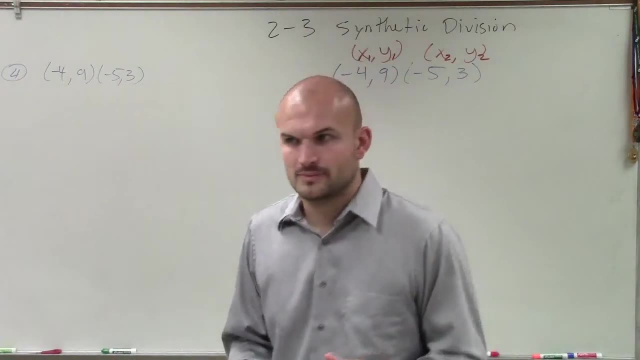 x1, y1, x2, y2.. All it is is a way to label them. The one and the two don't have any numeric value with the points. They're just a way to label them. Okay, Now let's go ahead and take a look. 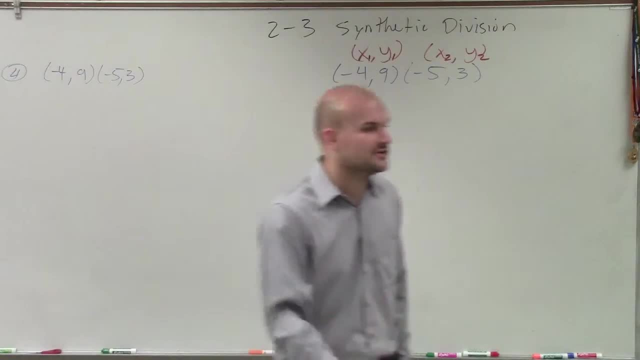 at the distance formula. Now, this is something I've been trying to present to you that you're going to want to make sure you have written down, which we're going to talk more about on Monday as well, But if I want to find the distance between two points, 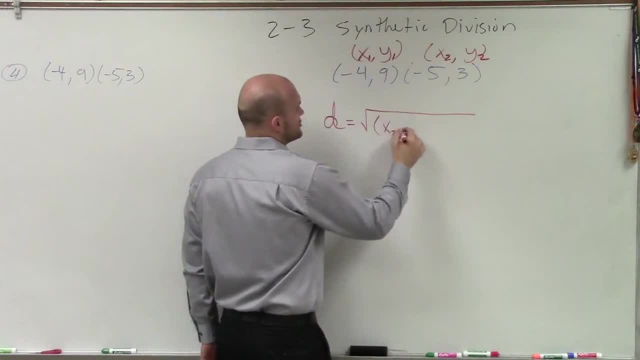 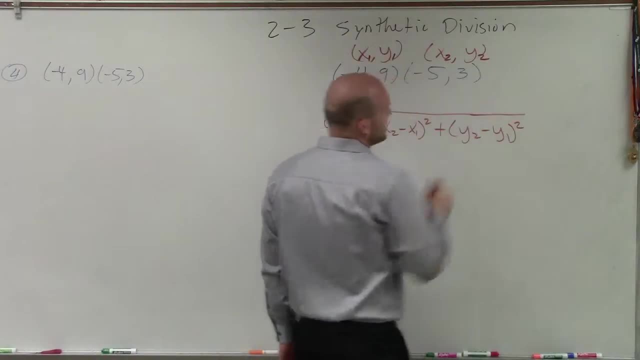 that becomes the square root of x2 minus x1 squared plus y2 minus y1 squared Again, don't worry so much about this formula. We're going to talk more about where it comes from again, But right now I just want to make sure. 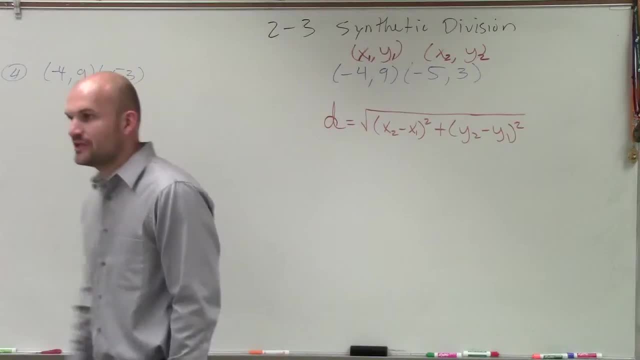 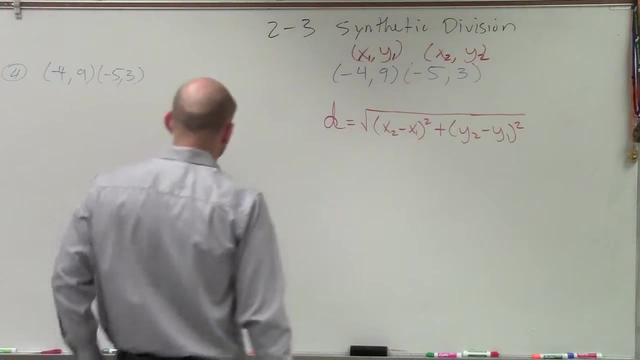 that everybody has that formula in their notes so they can apply the problems that we're going to be working on today. Because in label now, what we're simply just going to do is- let me give you guys an example, If you guys remember, 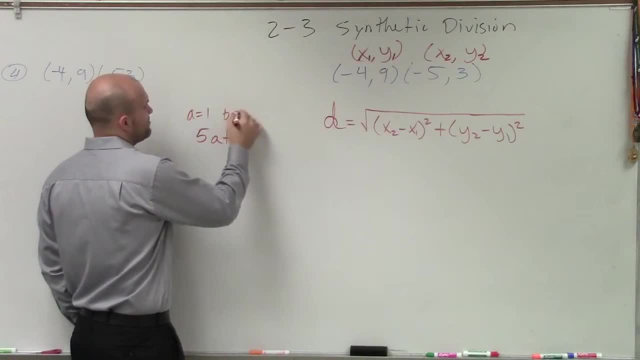 if I gave an expression 5a plus b and I said a equals 1 and b equals 3, what do you do with the 1 and the 3?? Do you remember what you do with 1 and the 3?? 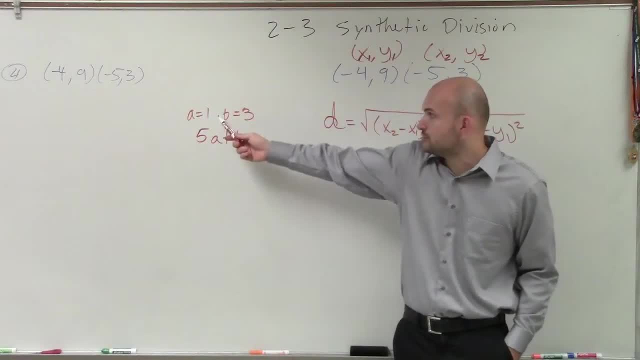 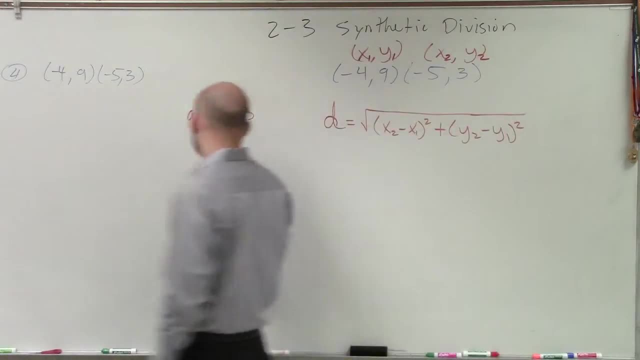 If I said: simplify or evaluate this, what would you do with 1 and the 3?? You'd plug it in for the a and the b, right. Good If I said: f of x equals x plus 5, and then I say: fine, f of negative 1,. 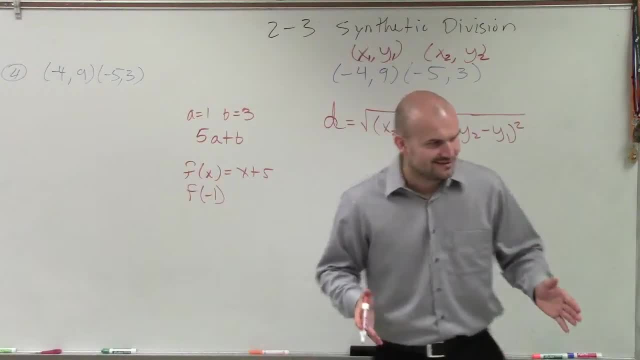 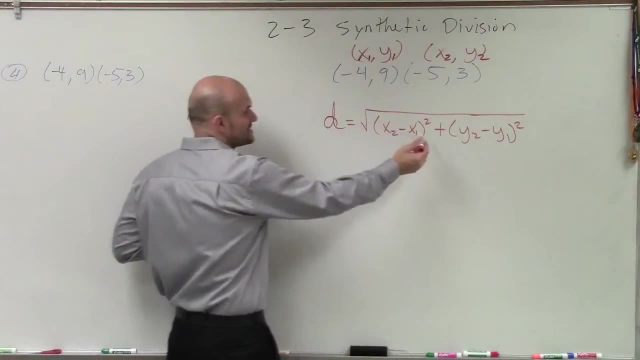 does anybody remember a function of what you do? Yes, Plug it in, right. So, ladies and gentlemen, if I say the distance is x2 minus x1 squared, plus y2 minus y1 squared, and I said: hey, here's two points. 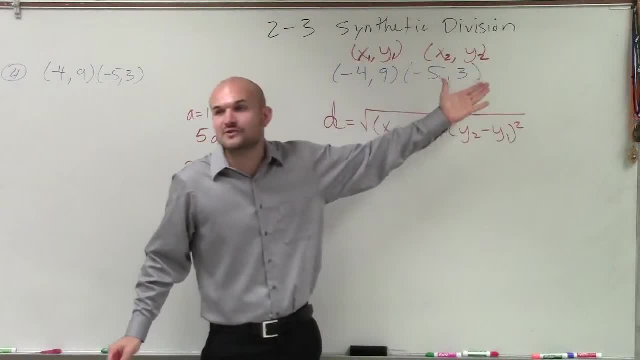 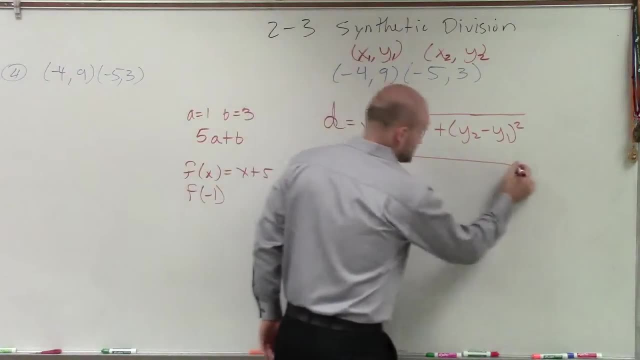 you label them x1, y1, x2, y2,. what do you think you can do with those points? Plug them in. Plug them in exactly. So therefore I have: d equals the square root of x2, which is negative 5,. 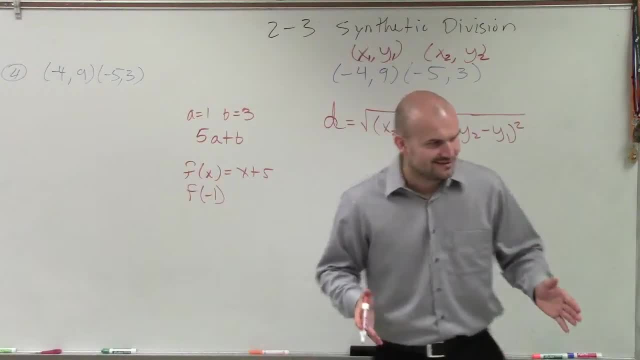 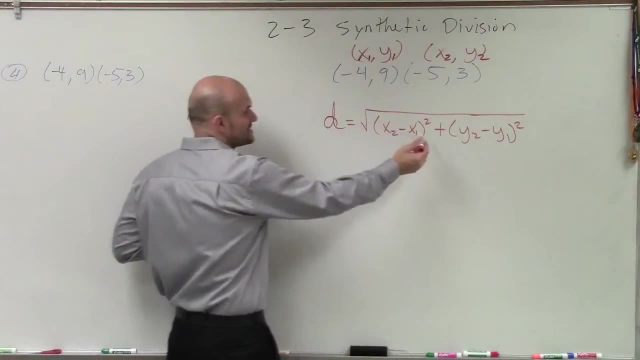 does anybody remember a function of what you do? Yes, Plug it in, right. So, ladies and gentlemen, if I say the distance is x2 minus x1 squared, plus y2 minus y1 squared, and I said: hey, here's two points. 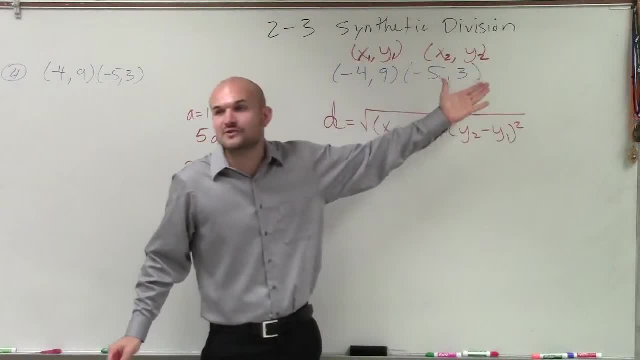 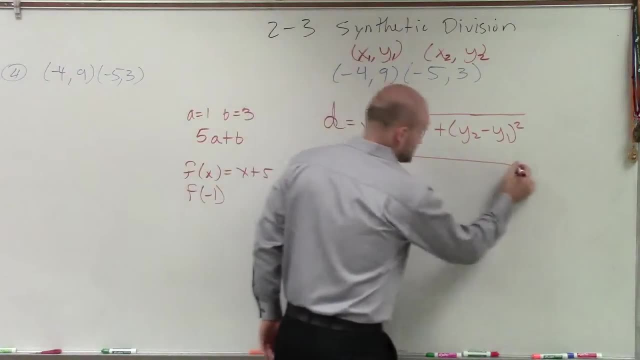 you label them x1, y1, x2, y2,. what do you think you can do with those points? Plug them in. Plug them in exactly. So therefore I have: d equals the square root of x2, which is negative 5,. 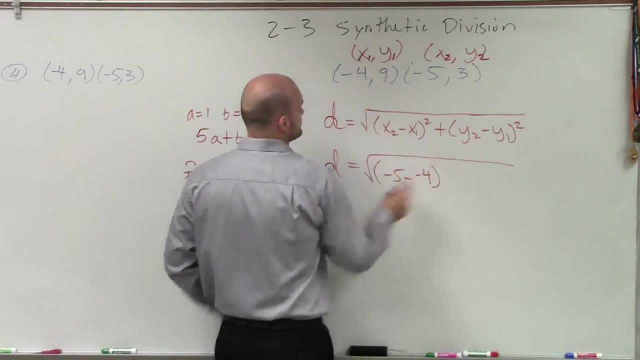 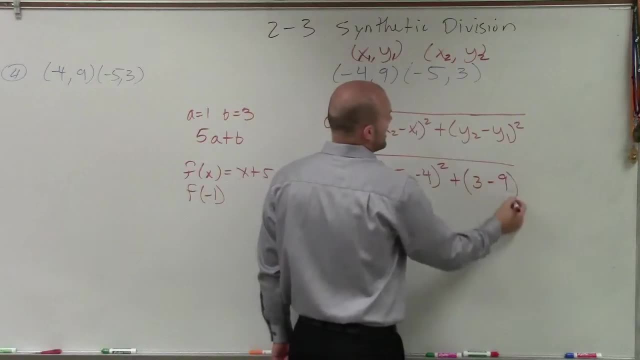 minus x1,, which is a negative 4, squared. plus y2,, which is 3,. minus y1,, which is 9, squared. Now we just need to do our mathematics, And this is where a lot of students might get caught up. 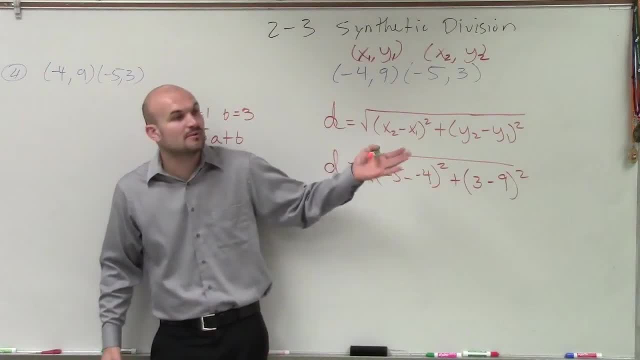 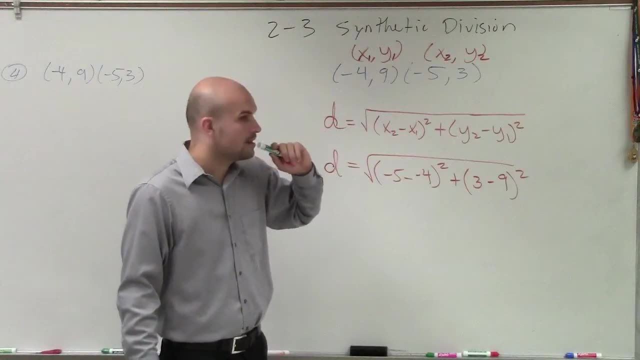 We have negative 5 minus a negative 4, alright. Remember, when we have a double negative, yes, That's a positive. Yeah, that's what my teacher called it. add the opposite. Yeah, you add the opposite, it's like a double negative. 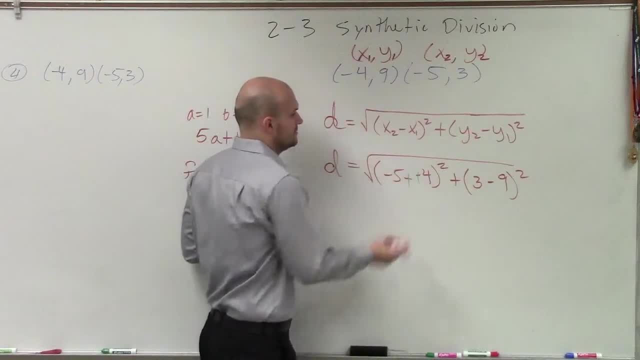 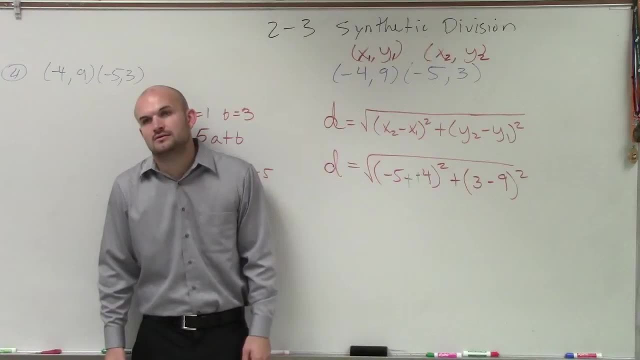 So what you get to say is like: this is like: Put a line through it, Yeah, it just turns into an addition problem. So therefore, I really have negative 5 plus 4, which is a negative 9.. Negative 5 plus 4 is: 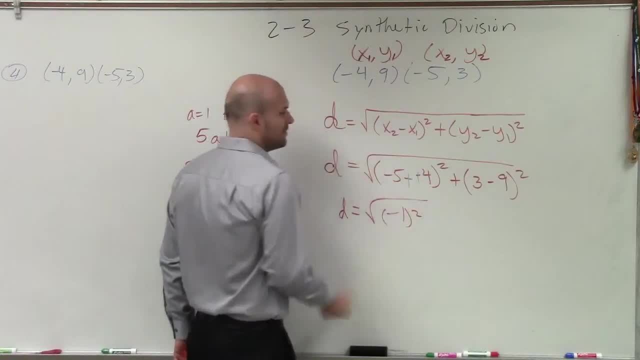 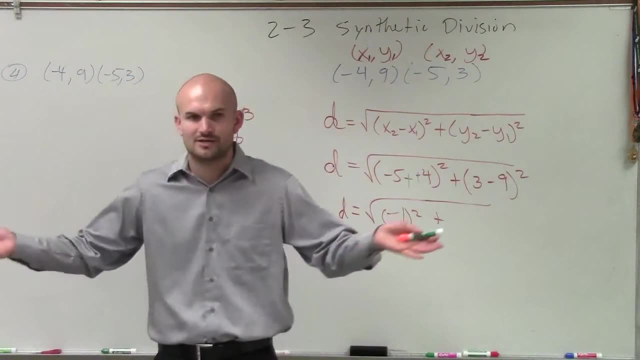 Negative 1.. Negative 1 squared Then plus 3 minus 9, you have 3 dollars. you owe somebody 9, now you show up for lunch and you have how much money You still owe somebody. 3 minus 9 is. 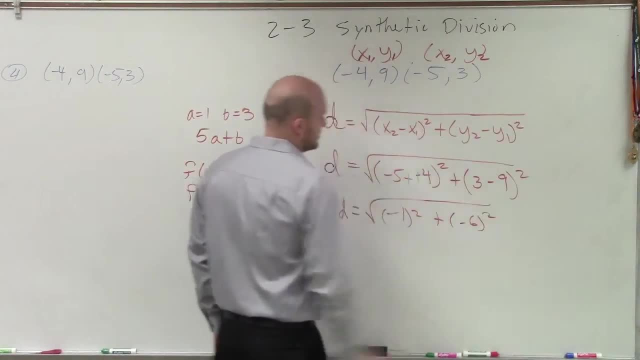 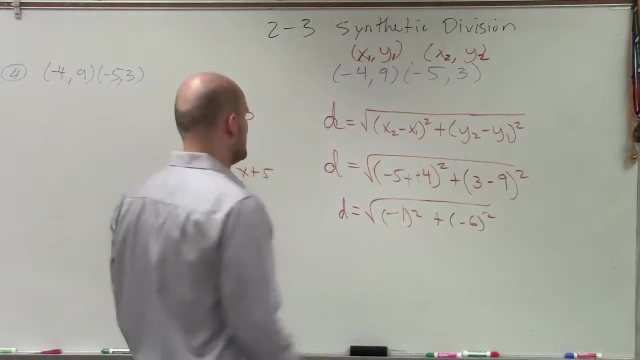 6. Negative 6.. So now we have the square. Remember, squaring is multiplying a number by itself. So negative 1 times negative 1 is going to give you a Positive 1.. Positive 1.. And then negative 6 times negative 6 is a. 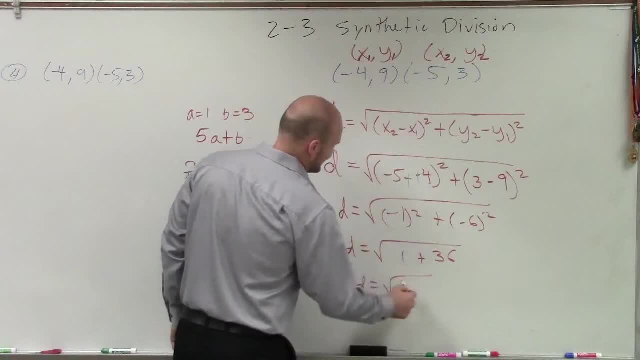 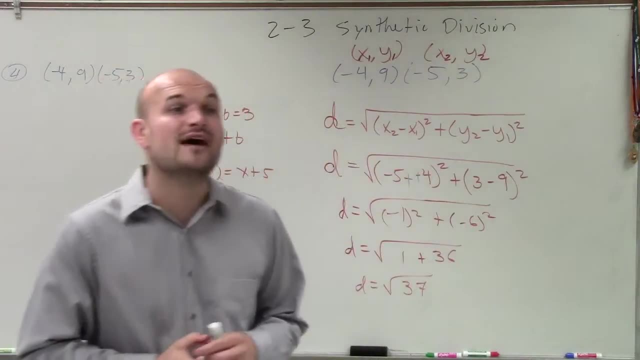 Positive 6, or positive 36. And therefore your final answer is going to be a square root of 37.. Notice, ladies and gentlemen, first of all, how I applied the order of operations Right Once we evaluated this.